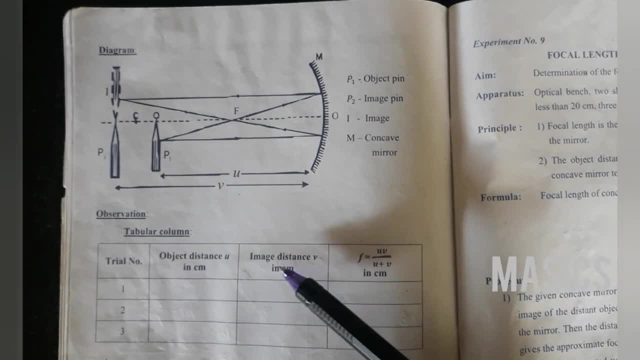 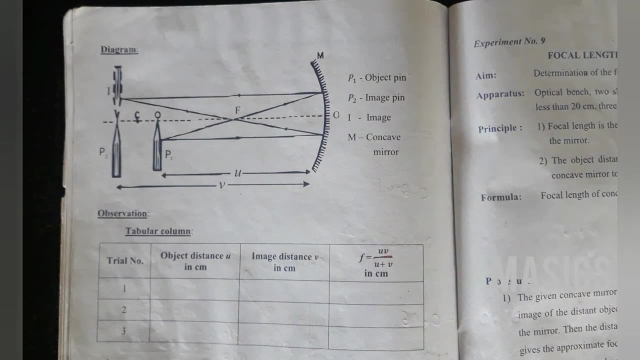 Object distance U In centimeter. Image distance, V in centimeter. So first set the object distance and find out the image distance and enter into the formula So we get the focal length of a concave mirror. Okay, yes, let us go to the experiment. 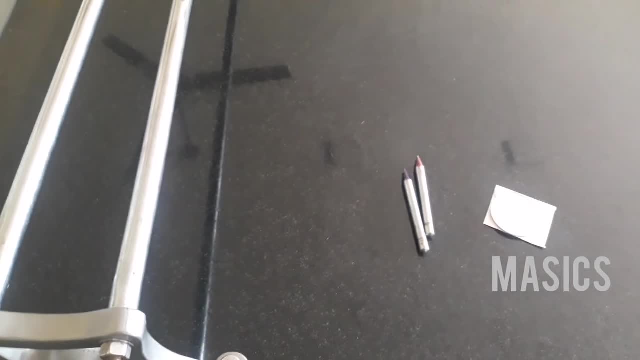 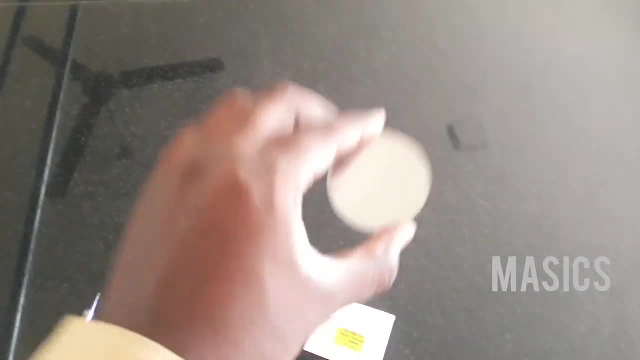 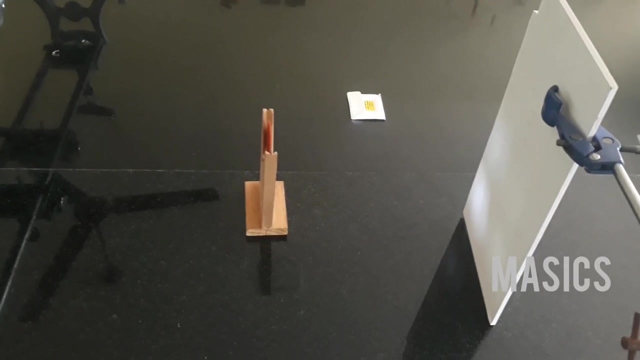 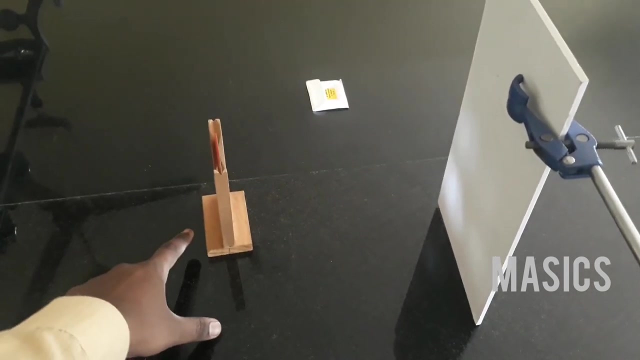 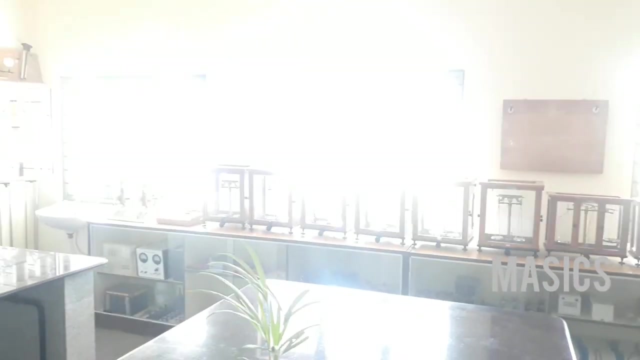 Apparatus required for this experiment: Optical bench, Two pins And concave mirror. Okay, so this is the concave mirror. Before start the experiment, first you find out the approximate focal length of the concave mirror. Okay, this is the mirror stand. I set the mirror like this and this one is the screen. So observe the window guys. Yeah, this is the window. Entire the window image is formed on the screen. Clear image. 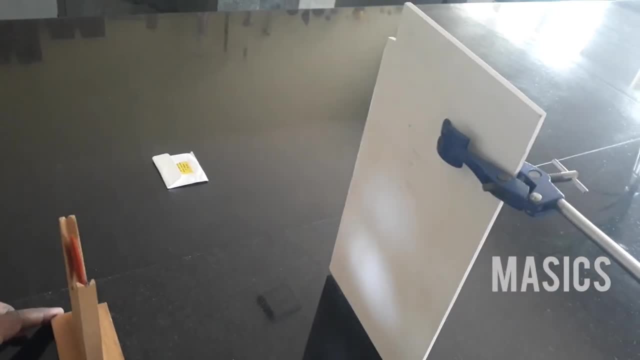 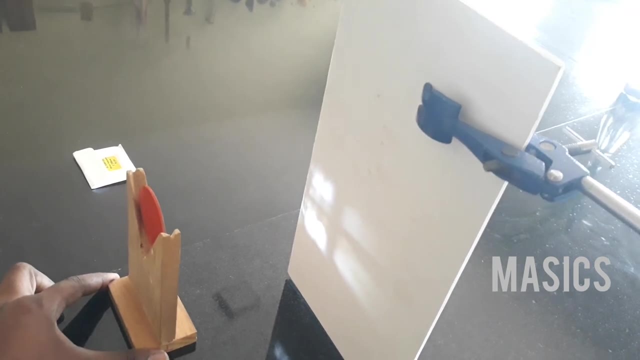 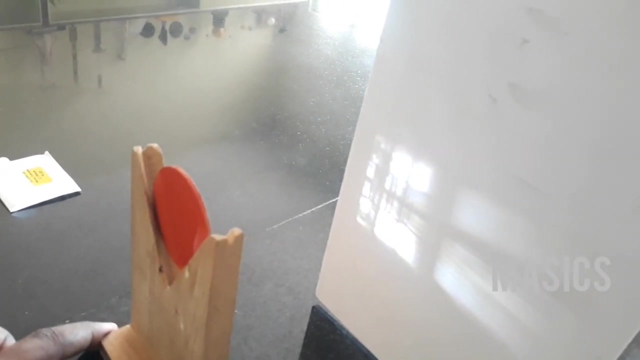 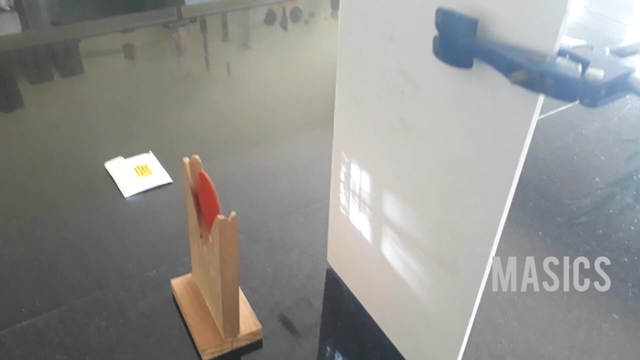 Listen here. How, sir? Listen here. So move the concave mirror towards the screen. Observe the screen, guys. The image is forming. Yes, see, now The clear image is formed. Is it right, When you get the clear image, measure the distance between the screen and the mirror? 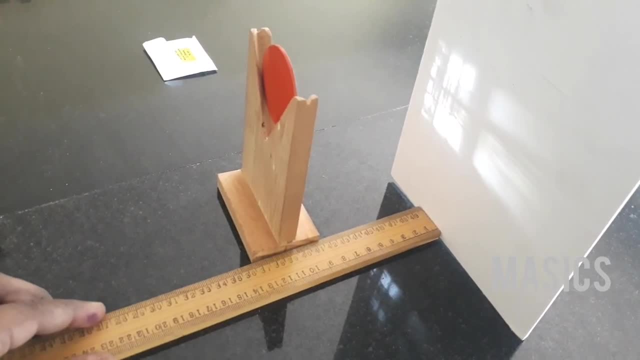 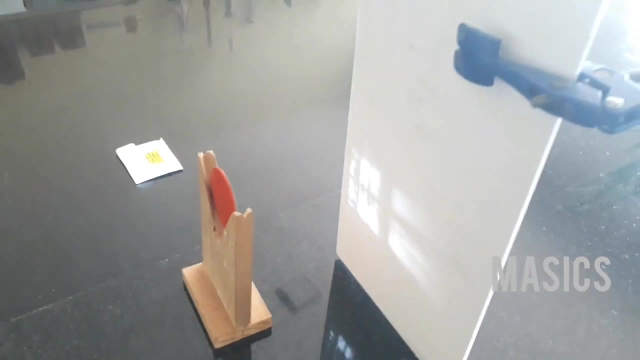 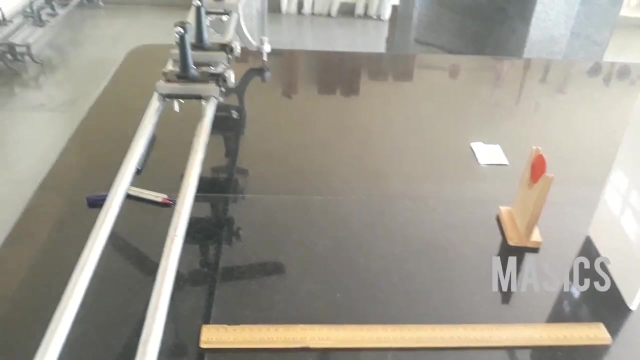 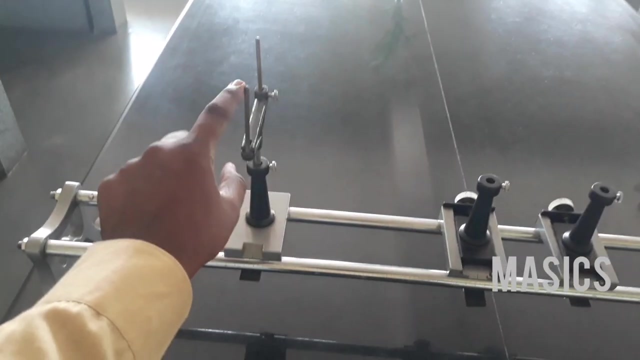 Like this. See Exactly at the center: 10 centimeter. The approximate focal length of this concave mirror is 10 centimeter. We have to prove this practically. Let us, we are going to start the experiment. This is the optical bench. This one is the lens holder or mirror holder, The first one taken as object pin. This is the lens holder or mirror holder, The first one taken as object pin. This is the lens holder or mirror holder, The first one taken as object pin. 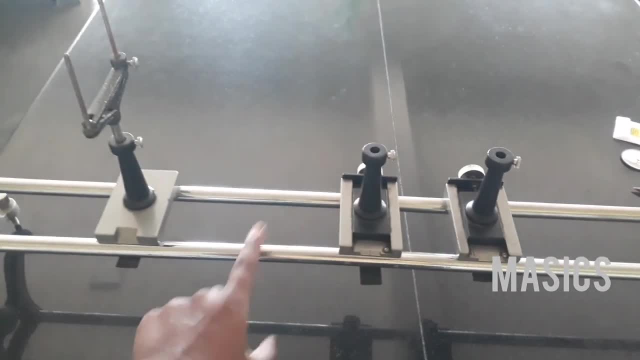 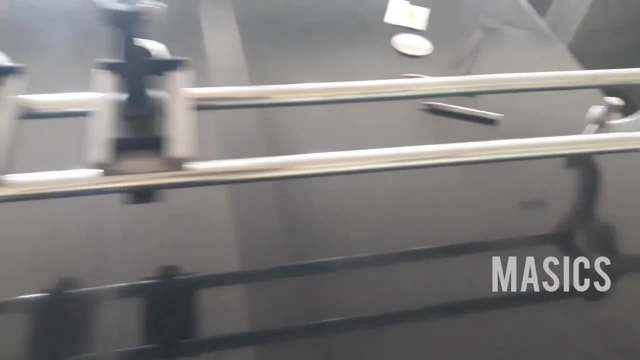 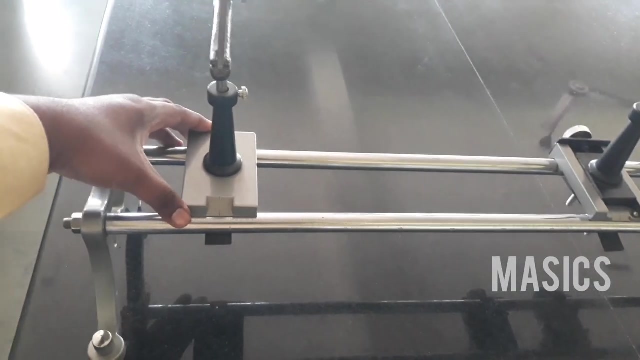 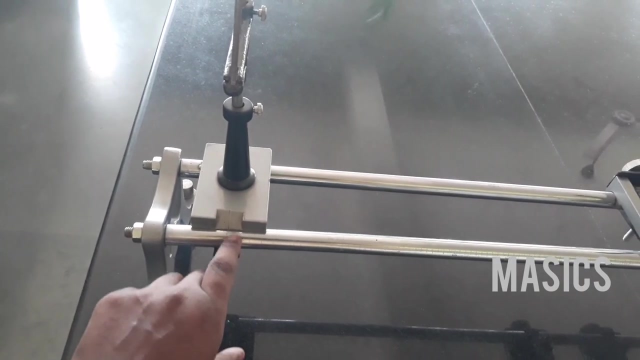 And the second one, taken as image pin. Okay, In optical bench, one meter scale is there. So this is the initial point 0 and this one is the final point 100.. Okay, Exactly at the point 0, you place the mirror holder like this. Okay, So, exactly at 0 centimeter, you place the mirror holder and fix the mirror. 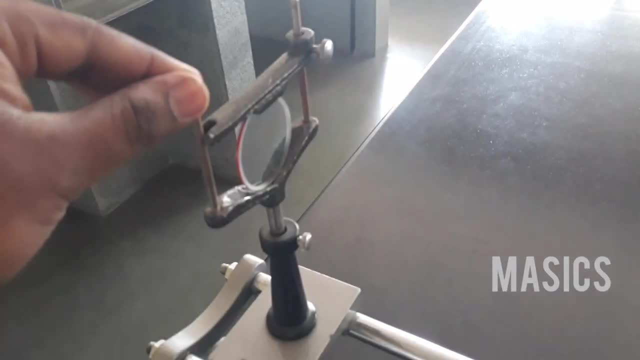 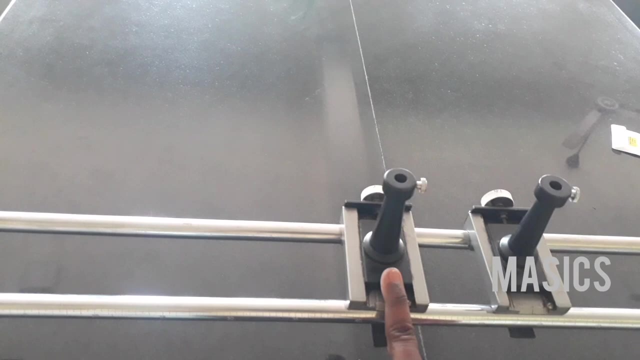 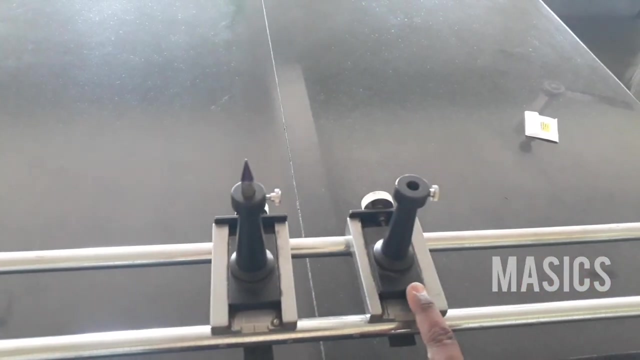 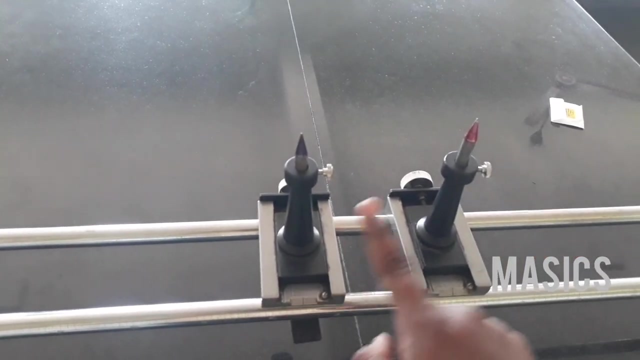 See, now I fixed the mirror. So fix the mirror like this. After that, take two pins, Okay, So, this one taken as object pin and this one taken as image pin. Okay, So, first one object pin and the second one image pin. 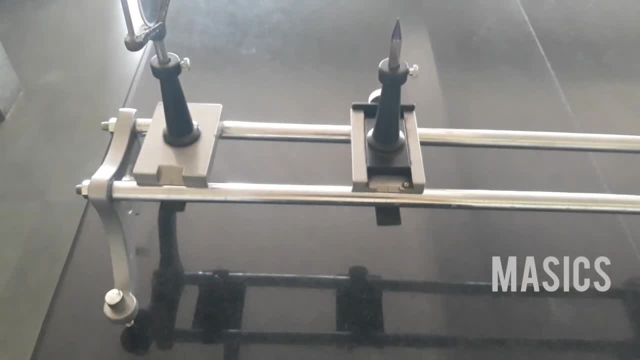 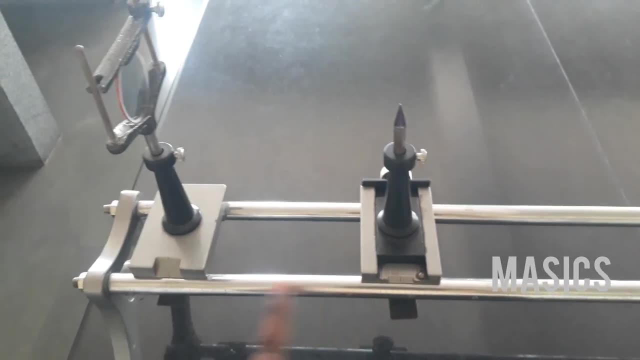 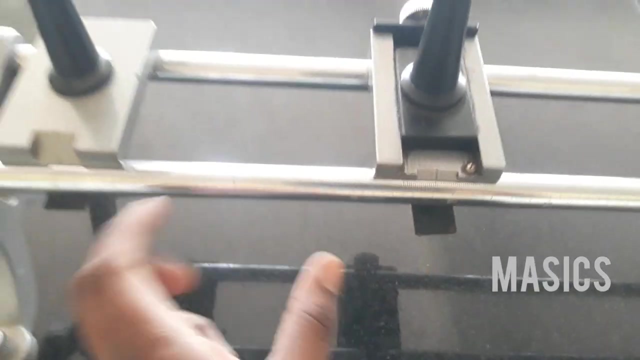 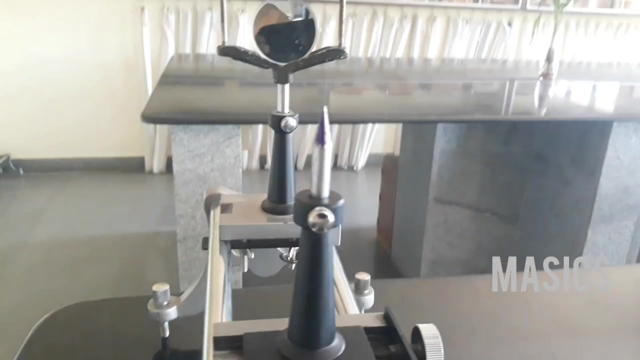 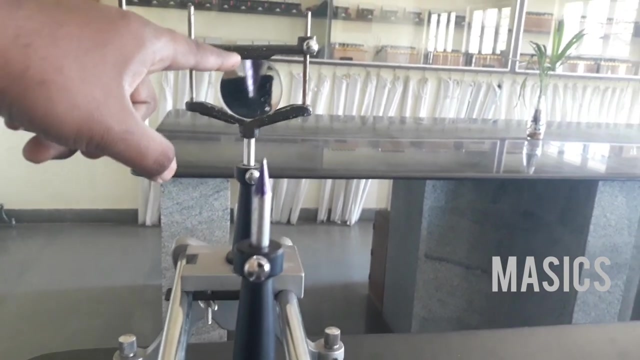 Okay, So first one object pin and the second one image pin. Now set the object distance. This is the concave mirror and this one is the object pin. The distance between the mirror and the object pin will be taken as object distance. Okay, See 0 and here 19.. The object distance is 19.. Okay, Then see the concave mirror. The real and inverted image of this object pin is formed in a concave mirror like this: 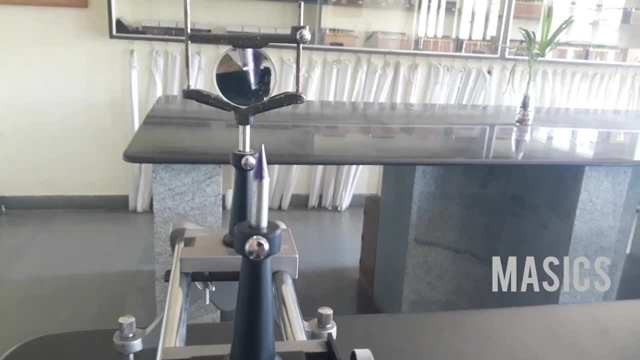 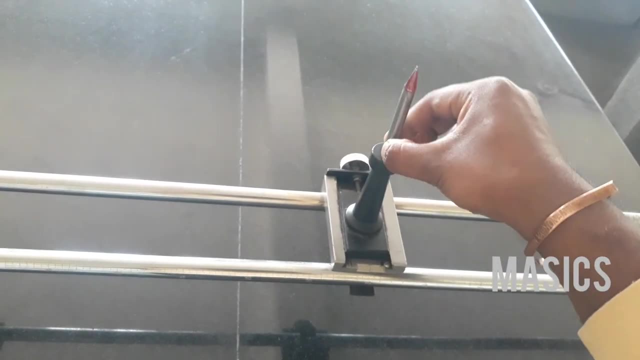 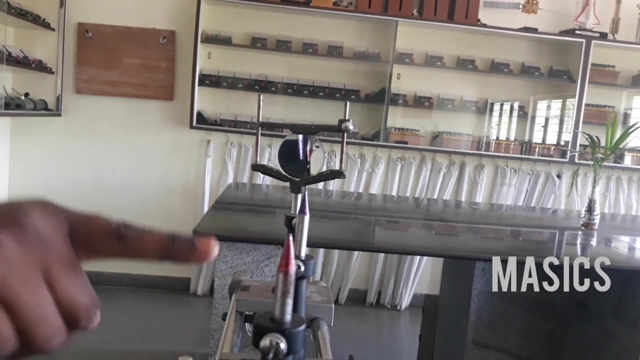 Okay. So next, what we do, sir, Very, very simple: Take a image pin. So, take a image pin and fix the image pin like this. Okay, Listen carefully guys. This blue color pin taken as object pin, This red color pin taken as a image pin. Okay, Observe the concave mirror. Both the pins inverted, image is formed, Is it right? 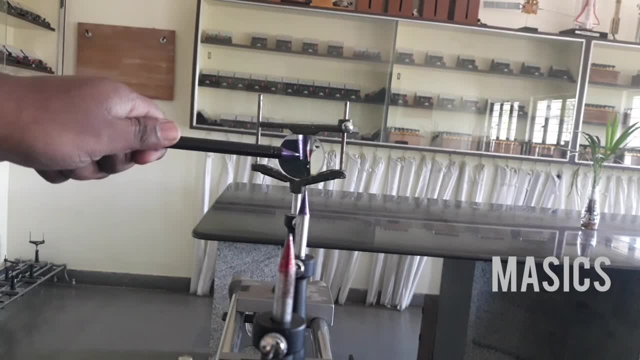 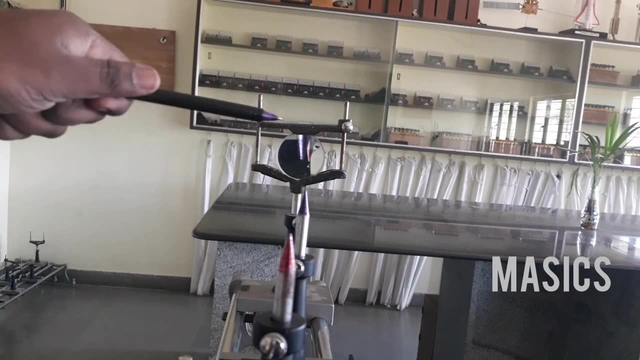 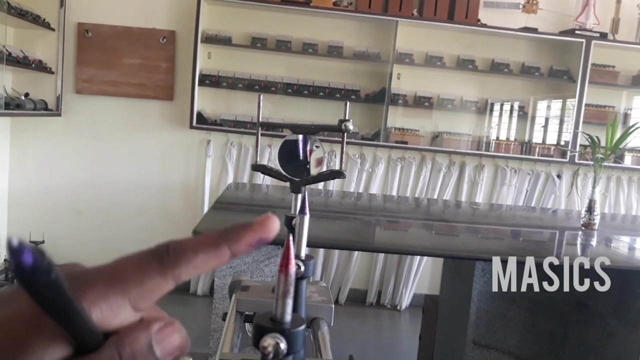 Okay, So object pin: inverted image and image pin inverted image. now neglect the image pin inverted image. red color formation: neglect that, okay. what we do next? yes, object pin inverted image tip. real image pin tip. you need to coincide without parallax. how to do, sir? yes, 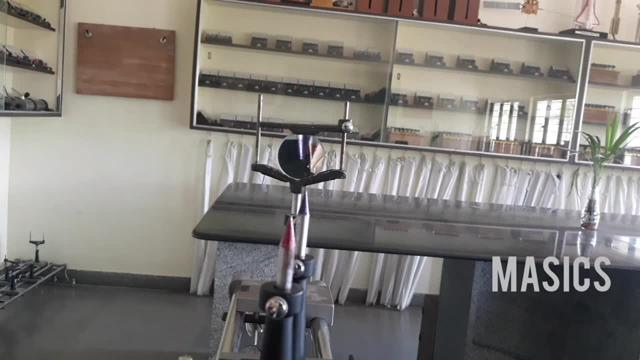 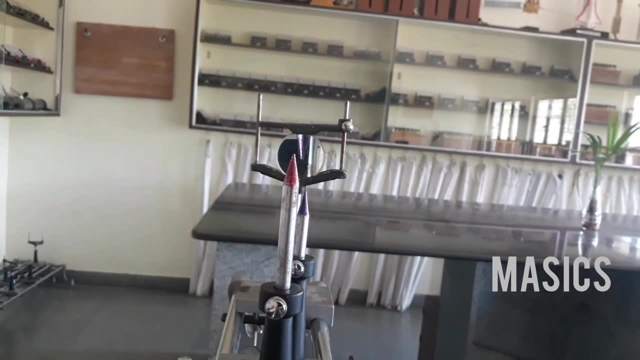 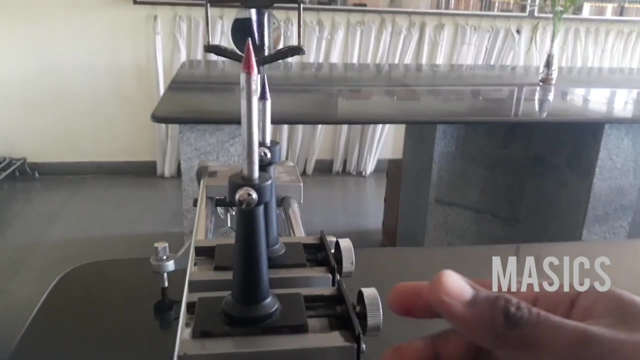 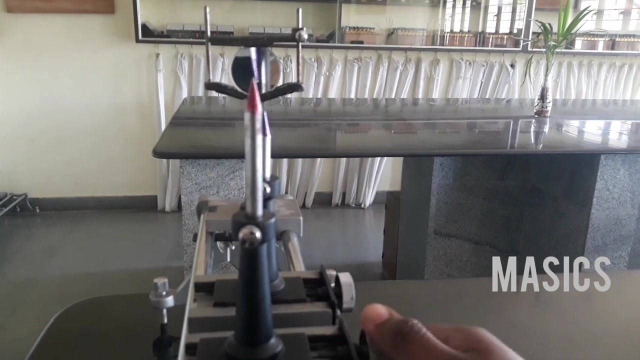 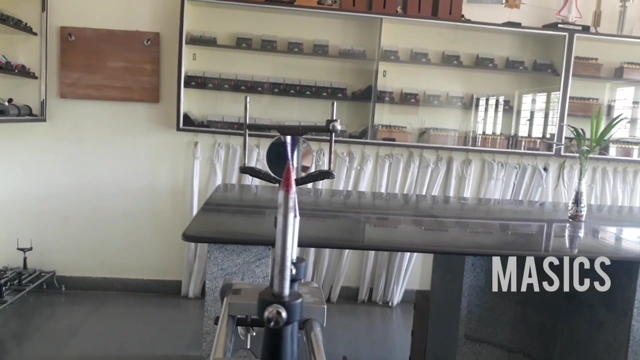 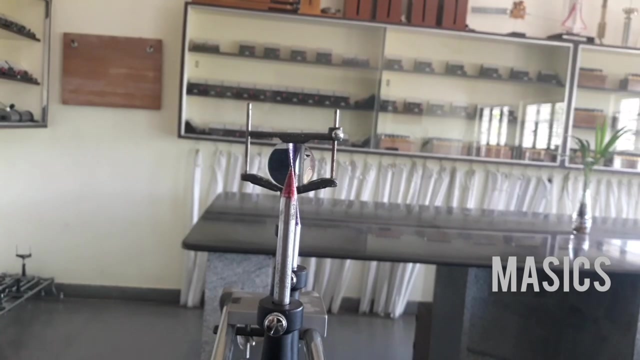 move the image pin like this: okay, so after that increase the height of the image pin like this: okay, see, now nearly coincide at the either. so after that operate the knob. okay, so in knob ideal. ah, so operate this knob like this: yes, now see both the object pin inverted image and the real pin image tip. both are coincide each. 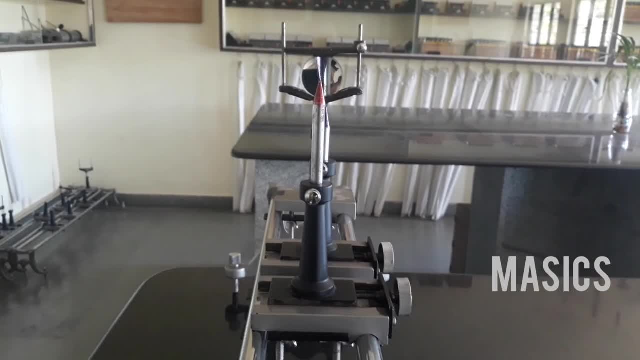 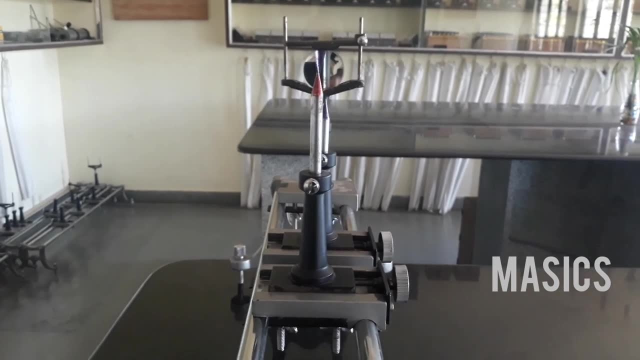 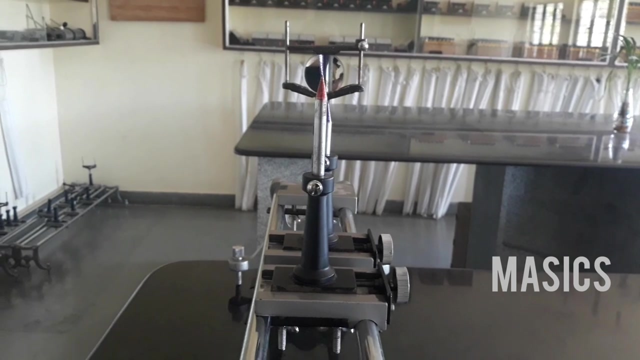 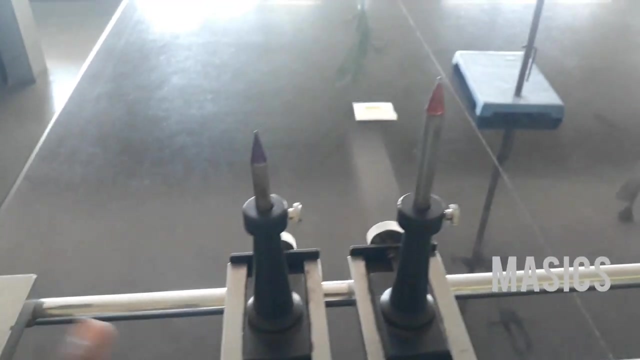 other. so after coincide like this, just move your high little bit right and left. see both are moving together, is it right? so this way, after focusing both, the tips will coincide without parallax coincide. take the image distance, okay, from mirror to the object pin object distance from mirror to 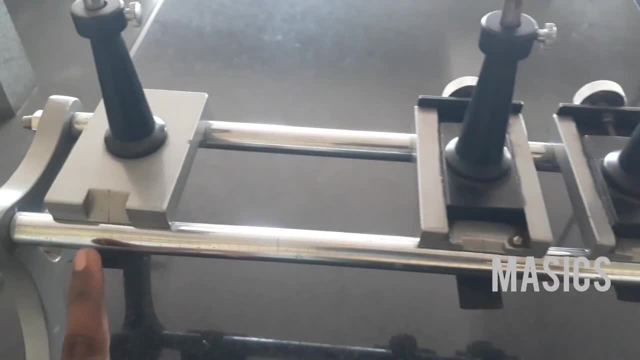 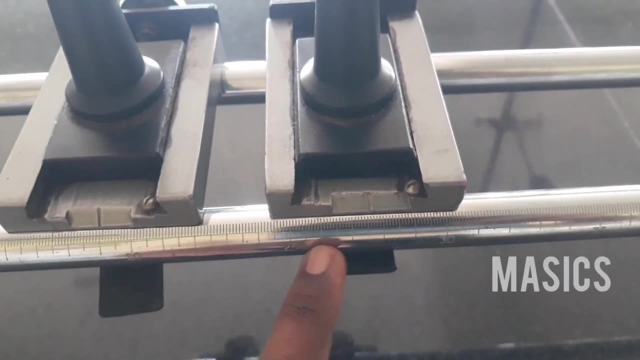 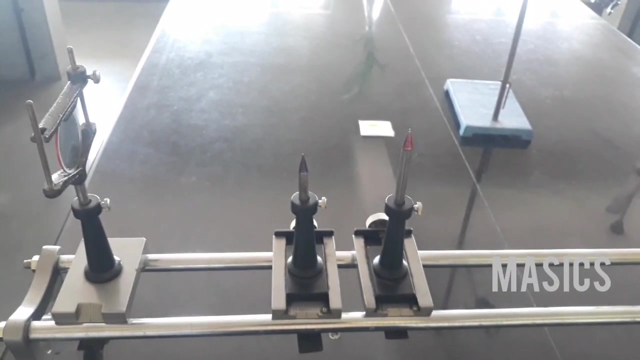 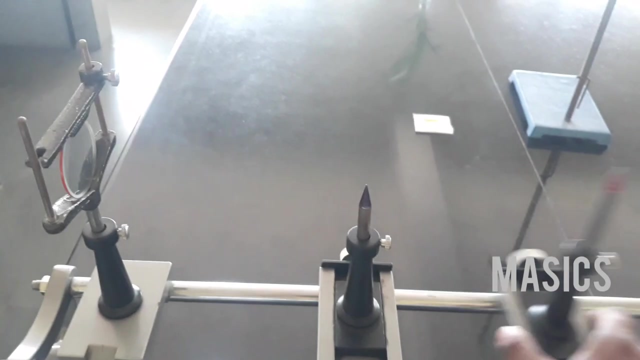 the image pin. image distance. here zero is there. so what is the image distance? image distance is 25, 26, 27, 27.5. image distance is 27.5. enter into the tabular column and calculate the focal length using a formula. second trial: just change the position of the object like this again: inverted image is. 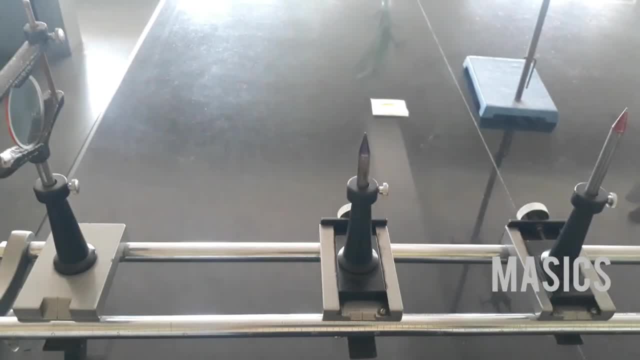 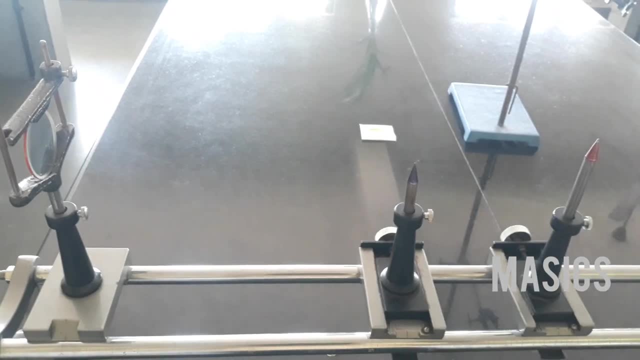 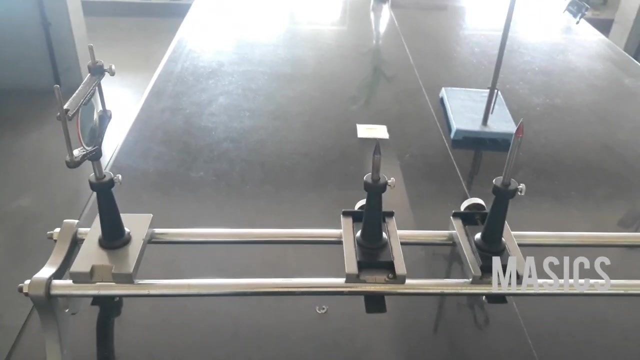 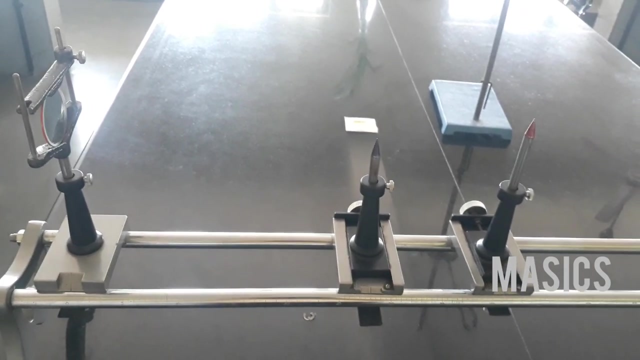 formed and coincide the two tips and take a image distance. third trial: again displace the object distance. again inverted image is formed. again coincide and take the image distance. that's all. so this is the way to find out the focal length of concave mirror. that's all let's. we are going to know the calculation part at last. calculation. 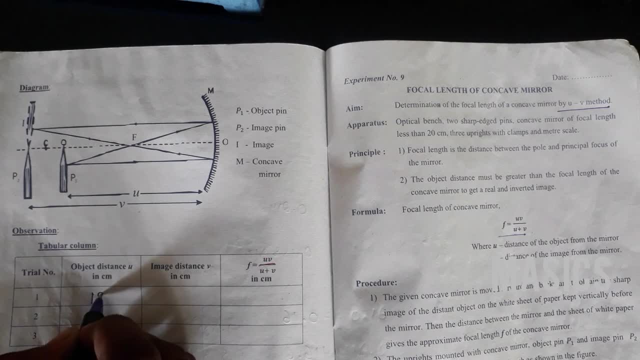 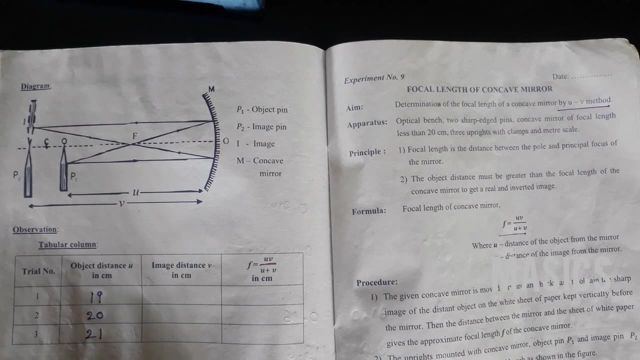 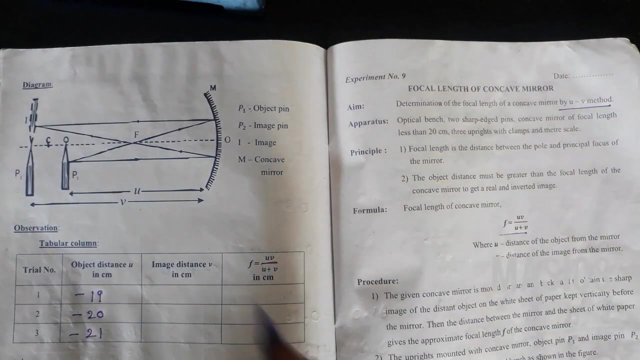 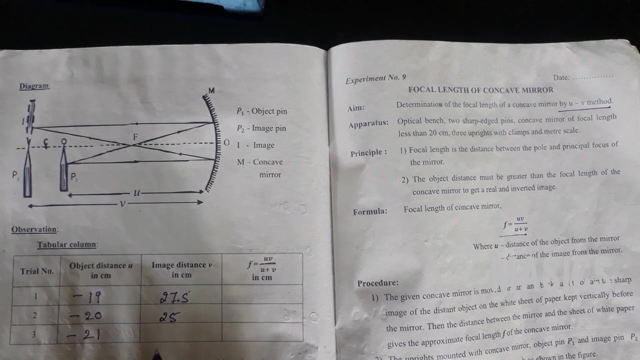 in first trial object distance: 19. second trial object distance: 20. in third trial object distance: 21 according to the cartesian sign convention, minus 19 minus 20 minus 21. next image distance: in first trial: 27.5. in second trial: 25. in third trial: 22.5. okay so. 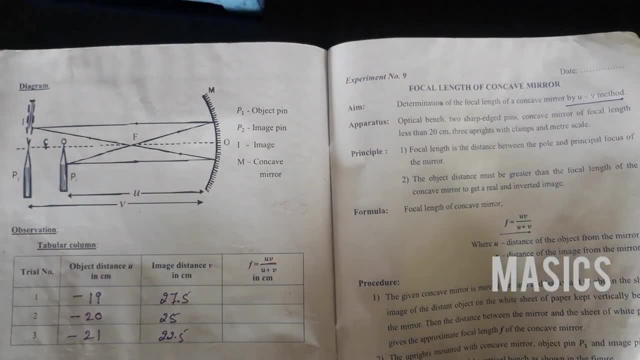 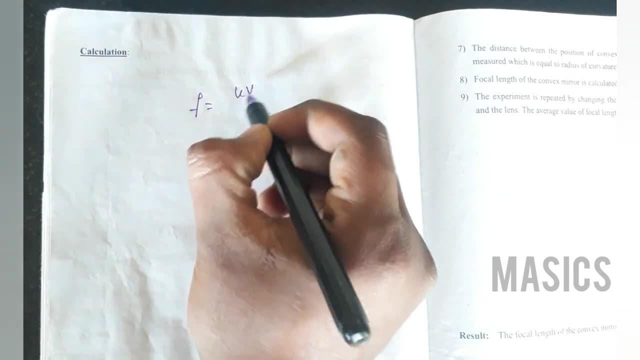 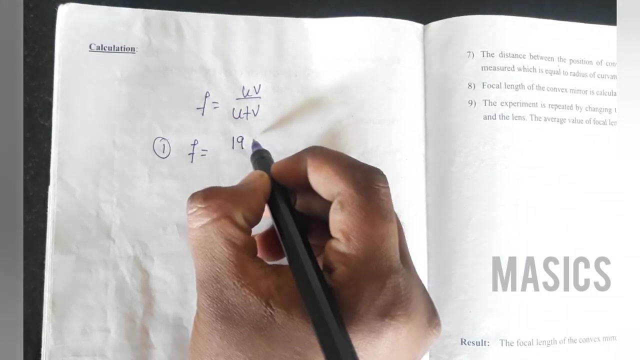 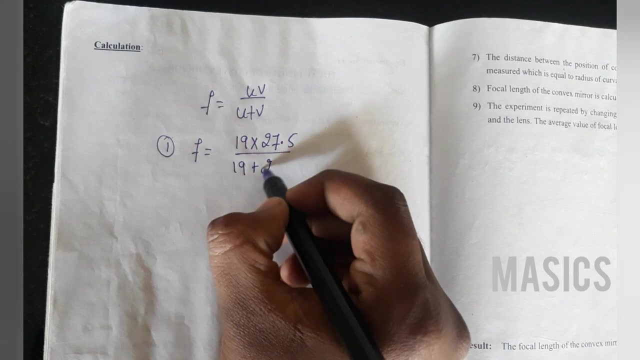 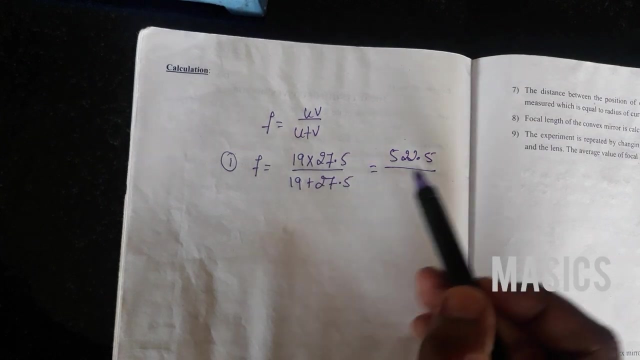 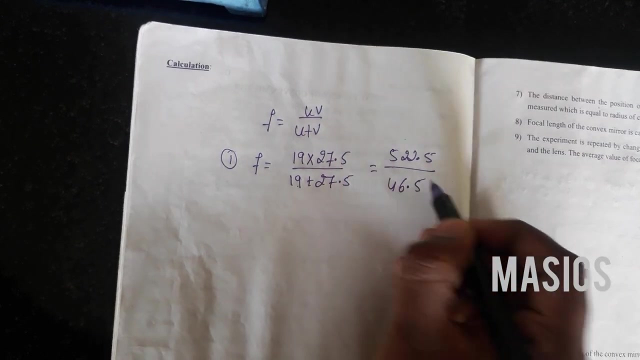 substitute this value into the formula. so what we get at last calculation formula: f is equal to uv divided by u plus v. okay, in first trial, u 19 into v. 27.5 divided by 19 plus 27.5. what is the answer? 19 into 27.5 is 522.5. 19 plus 27.5 is 46.5.